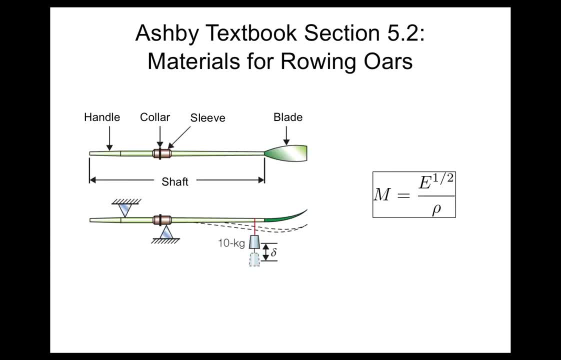 it's section 5.2 and it goes through materials for rowing ores, And so, if you remember, I've given you just a little picture of the schematic here. So we have the rowing ore we're assuming is a long beam and it's being loaded by a 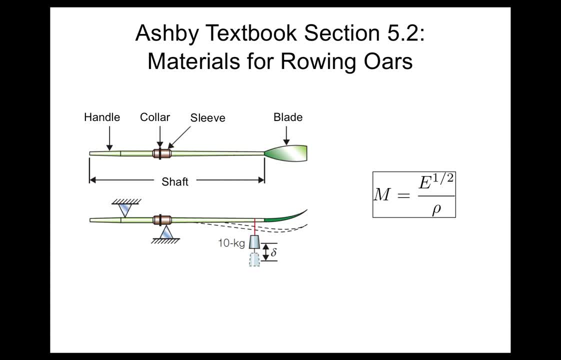 force, by a weight, and it has some sort of deflection. So we can look this type of problem up in in the back of the book. We're gonna- it's gonna be a beam in in bending, And so in this case we find that our material index is the elastic 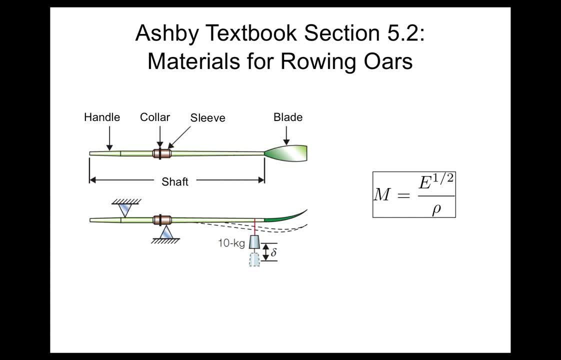 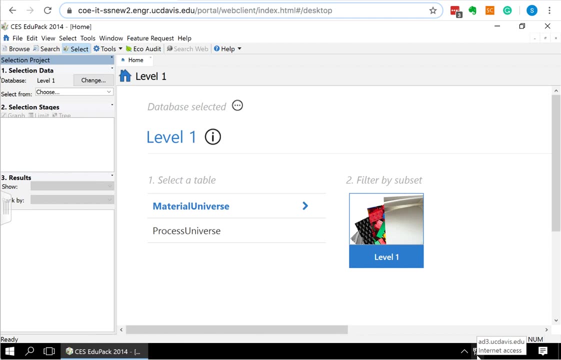 modulus to the one-half divided by the value of CES EduPack. So we're going to look at how to select this using CES EduPack. So, to select this using CES EduPack, we open up the software. I have already selected the level 1 database. 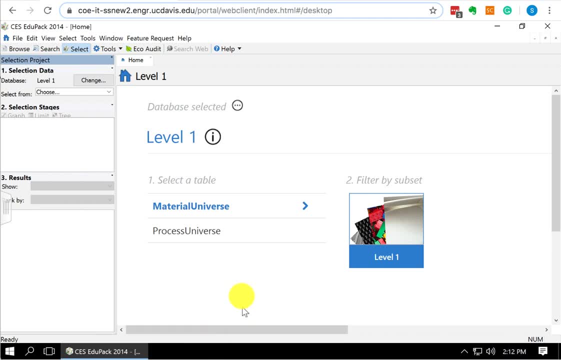 just for simplicity. but you could select one of the other databases And we select the material universe, level 1.. And so over here on the left, we get the selection project. So we're going to select the selection project and we're going to select the material universe level 1.. And so over here on the left, we get the selection project. 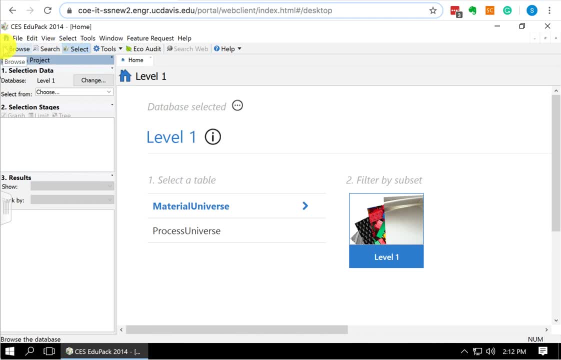 If you don't see that, you can just come up here. you know we can go. we have browse, search, We want select, We have level 1 and we want to select from again the material universe. So what we're going to do is we're gonna make a. 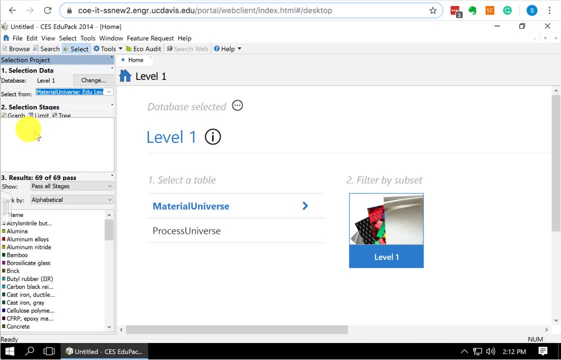 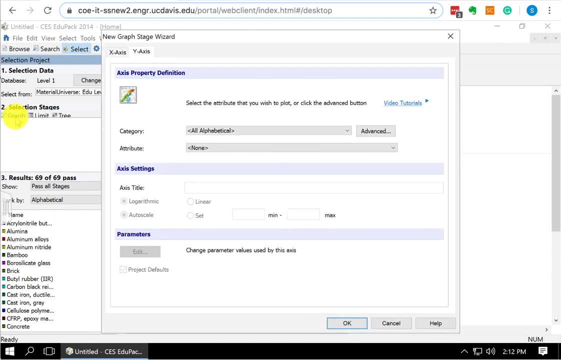 two-dimensional XY plot of our materials. So to do that, we go over here to now selection stages and we select graph. So now we are going to define the parameters that we want for our axes. Now we're going to go over here to our 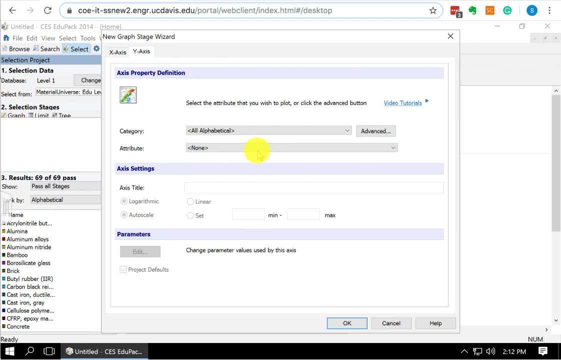 axes. So for the y-axis, we want this to be the elastic modulus. So I clicked category. It's going to be under mechanical properties, or you could look under all So mechanical properties, and then our attribute is going to be the Young's modulus, Remember. 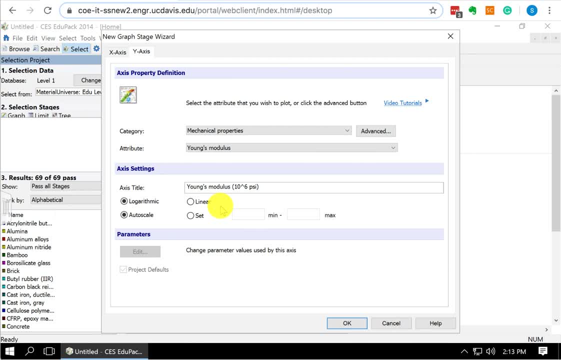 Young's modulus is another name for the elastic modulus. These are the same parameter. The x-axis we're going to set is going to be our density, So our category- we could leave them all here, if you want- Our attribute is going to be density. So when we've selected our x and our y-axis, 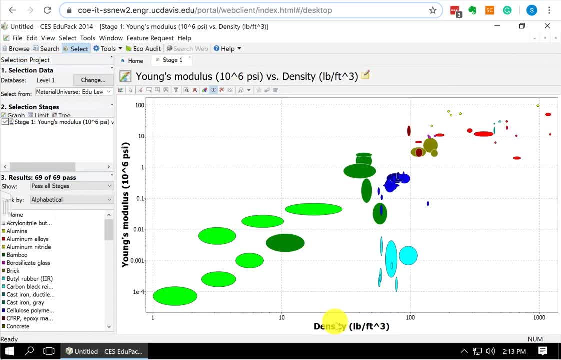 so now we can go down and we can select OK, And this creates an x-y plot of these two parameters. So you can see all these materials. We have 69 materials here and all of these materials are plotted. Now what we want to do is we want to draw in the line for our material index. 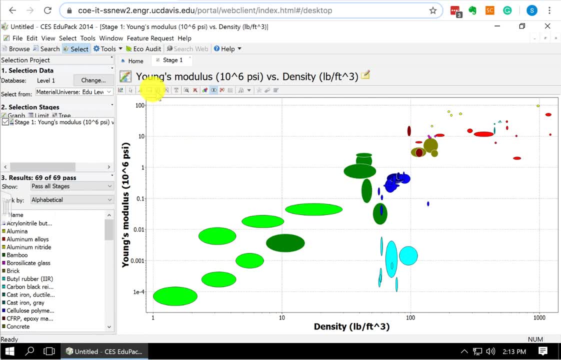 So to draw in that line, we come up to these little icons up here. We choose the one that's the gradient line selection. We select that one And here I'm going to enter the slope of my line. Remember, I take that elastic. 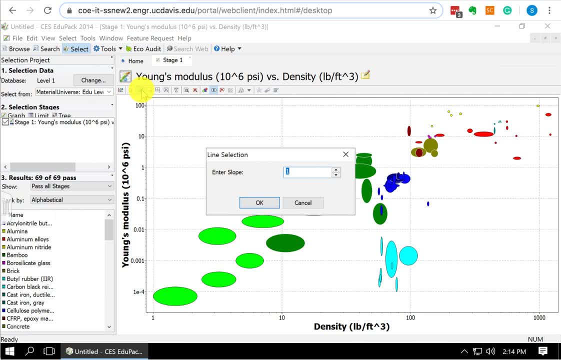 modulus, or I take that material index, you know e to the one, half divided by row. I take the log of both sides, I rearrange it and we find that our slope should be two. So we enter our slope and we 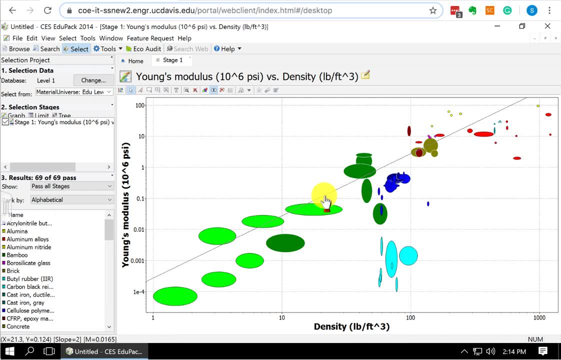 click OK And we see that our slope is anywhere on the plot and it draws in a line with a slope of two. If we come down here at the bottom, you can see where I clicked the value of x and the value of y. 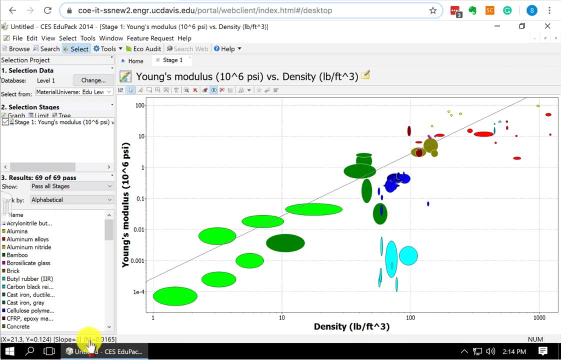 My slope again is two And we also can see here what are the value of our material index is. So here we see that that line, any point on that line, has a value of M equals 0.0165.. And so actually if I click on the line again and I move…. 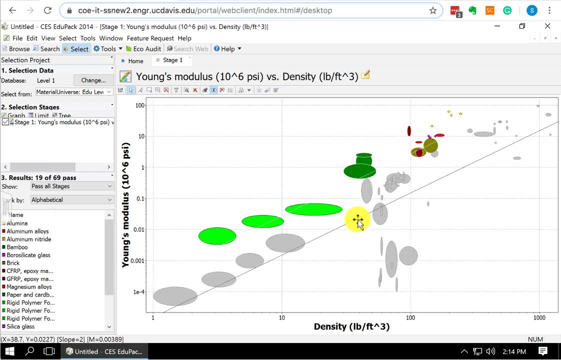 Sorry, Click on the line again. I move it down. we see that those values of m get smaller and smaller. So now I'm down to 0.001.. If I move my line up, m gets bigger and bigger and bigger, You know. so here we're already up to 0.02.. 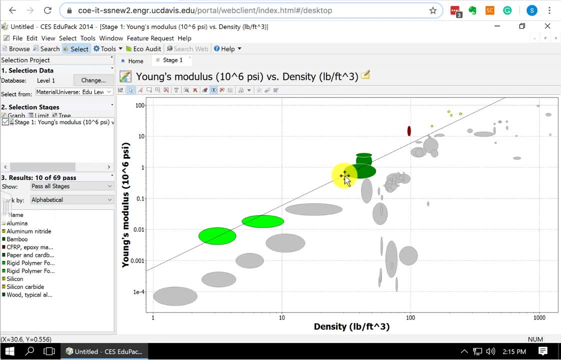 And so, if we remember from our problem, we specified that we want to maximize our material index. So we want to choose, draw our line to be the largest value of m. that still lets you know, maybe five or ten materials pass. And so we draw this line and we will put it here. And so what? the 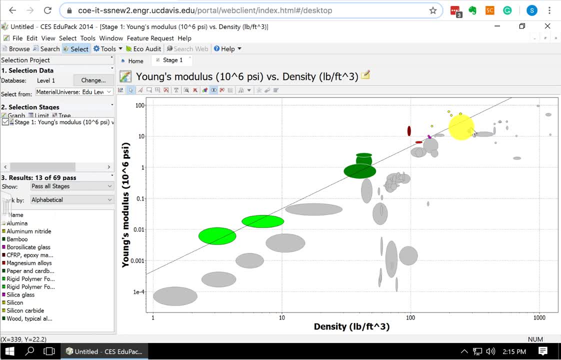 software does is it's selected to shade everything below the line in gray. So those are the materials that don't pass, that don't fit our criteria, And it shades in it colors in the materials above the line that are the materials that pass our criteria. So in this case it guessed correctly. 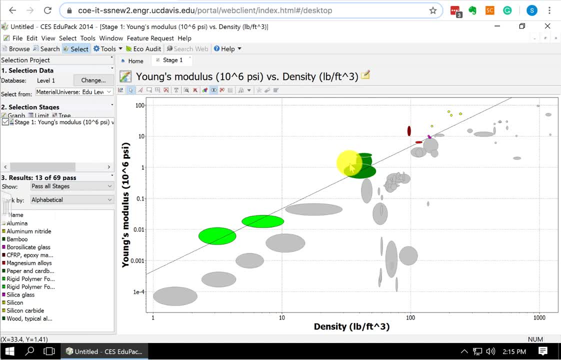 and it shaded the right side. We want to maximize our material index, So we want the ones above the line to be shaded. But if we were going the other direction, what we could do and we needed to minimize our material index and have these parameters, these materials down here, be shaded. 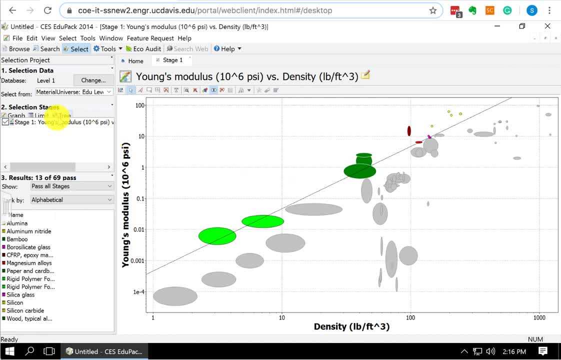 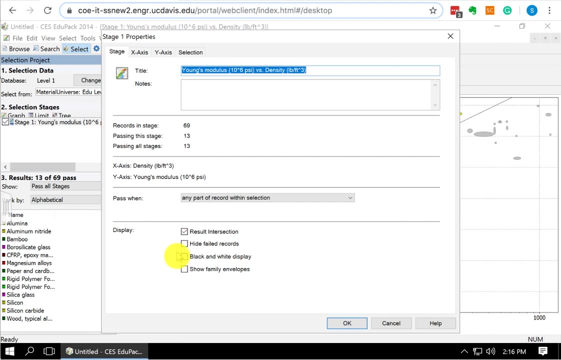 instead. Well, so what we can do is we can come over here to our stage Where we said stage one, Young's modulus, we right click on that and I edit my stage. So this gives me the opportunity to change my x and my y axis. You can also see, you know, if we want to hide some of 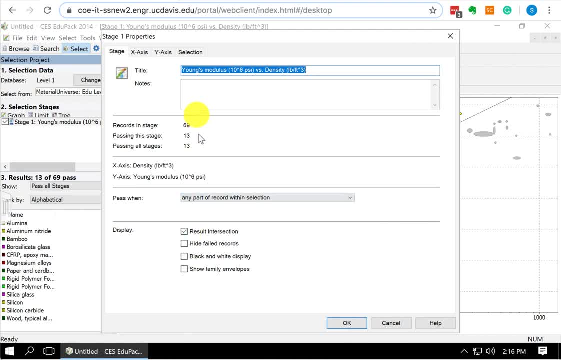 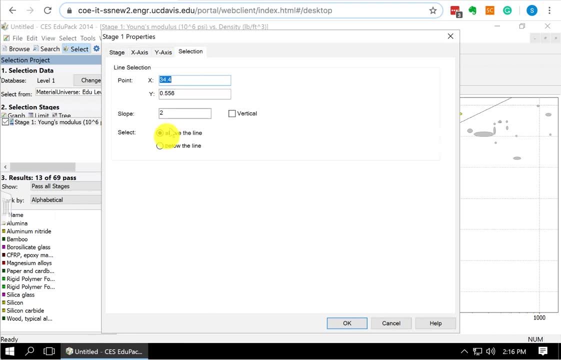 the materials that didn't pass. we can, we can do that, But we also up here, if we click on the top right, we can click on selection And this is where you can see I currently it's- I select things that are above the line. 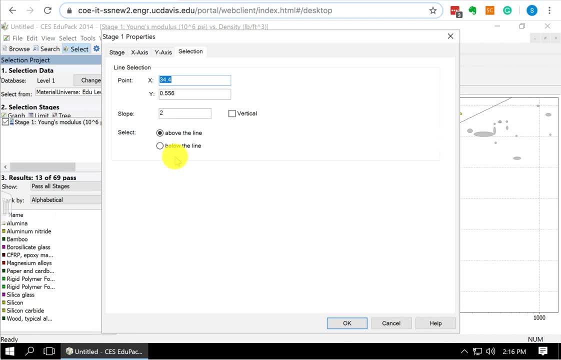 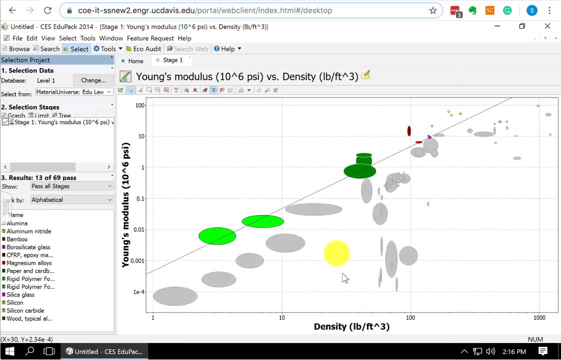 But if we needed it to be in the reverse, we could also select below the line. So, like I said, we'll leave it as above the line, But that's where you can change it if you need to, And so we've shaded. 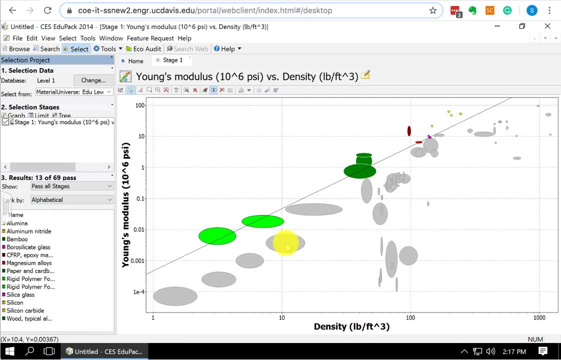 in all of these materials And so what we can do. you can see we have about 13 materials. If you want to get rid of a few more, we can go a little higher. We're down to 10.. Go a little higher. 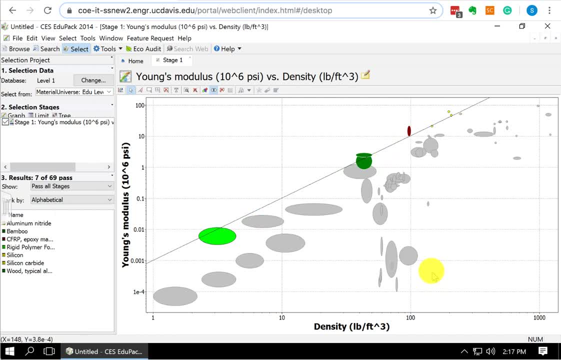 We're down to seven And so now what we can do is we can label these materials. So if we click on the material bubbles- so I'm just going to left click here- you can see this is rigid polymer foam. Up here this is going to be bamboo and wood along. Oops, don't want to change the line. Oops.